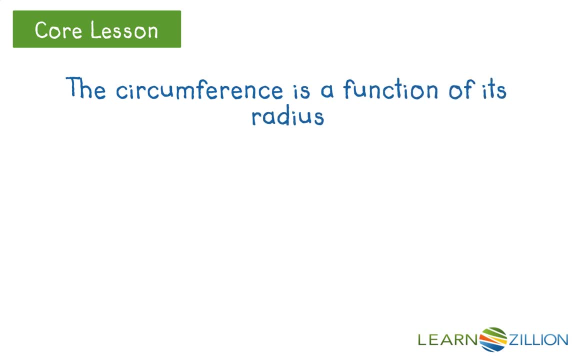 where we use the formula for circumference to interpret what our input and output values mean. The circumference is a function of its radius, which means that the circumference depends on the measurement of the radius. If my radius is 4 units, we use this as my input value. 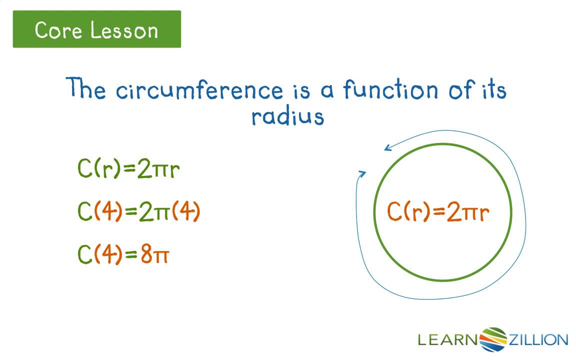 for the variable of r, And then, when I evaluate my function using 4 as my radius, I get c equals 8 pi. So what does this mean? It means that my output, or the circumference, is 8 pi when my input. 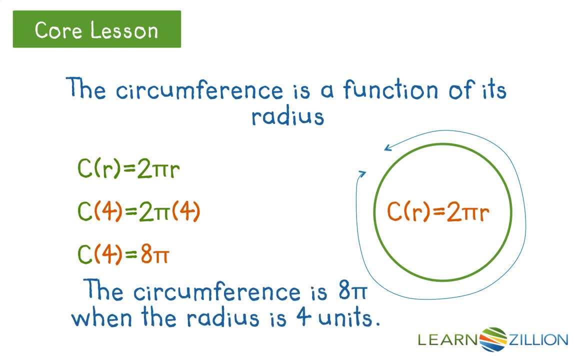 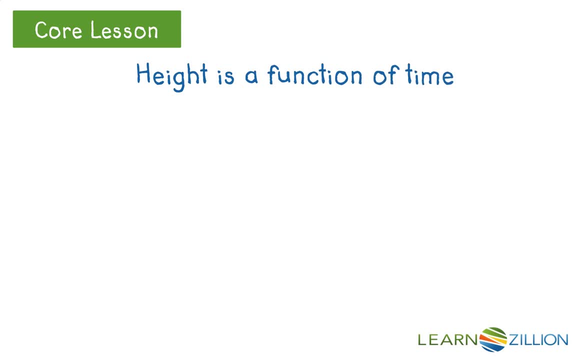 or the radius is 4 units. Let's look at something that's not linear, where I'm using the formula for height to interpret what my input and output values are. Height is a function of time, which means that the height depends on how much time has passed. 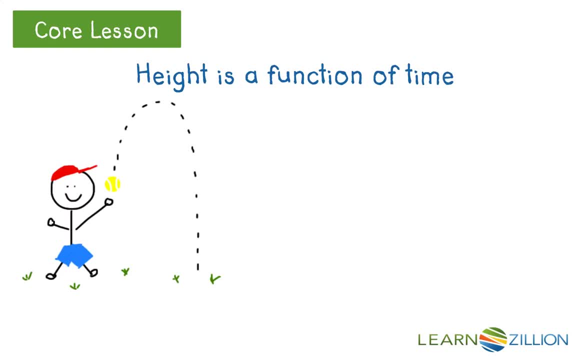 If you were out at the park and you threw a tennis ball straight up into the air, the formula to calculate the height of that tennis ball is: h of t equals negative 16t squared plus 29t plus 6, where the 29 is my initial velocity in feet per second, which means that's: 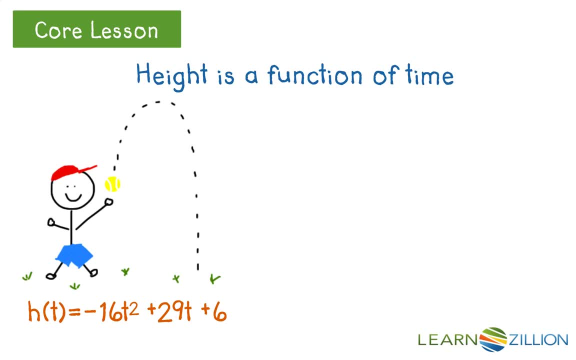 how hard you threw the ball up at the beginning. and then the 6 is my initial height of the ball and I'm assuming you're about 6 feet tall. If I want to know how high that ball is after one second, I just 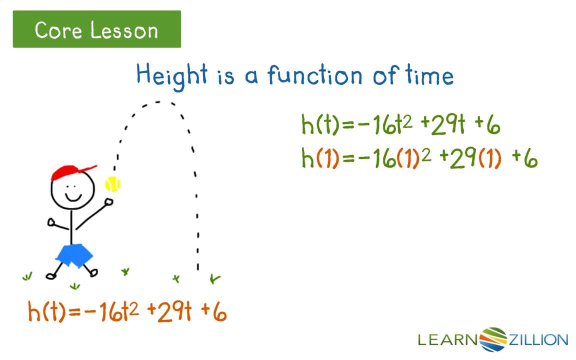 plug in 1 for my input of time or t. When I evaluate the function using 1 second as my time, I get h of 1 equals 19.. So what does this mean? It means that my output the height. 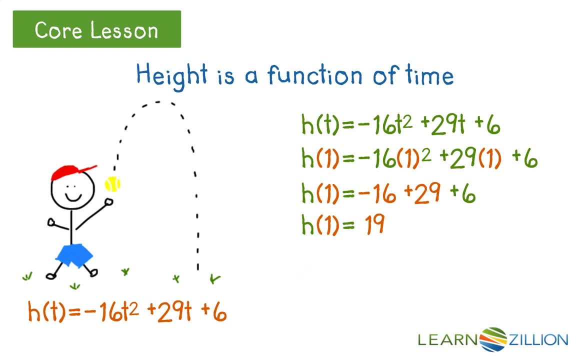 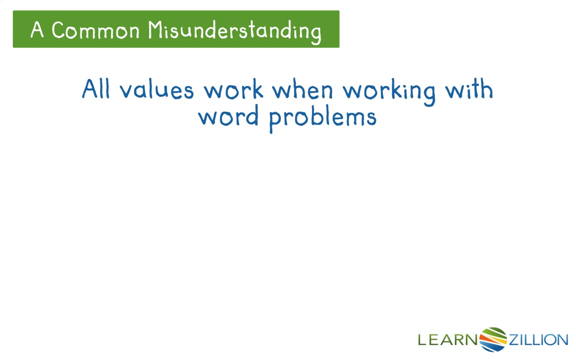 is 19 feet when my input t is 1 second, meaning 1 second has gone by. So the ball was 19 feet high after 1 second. A common misconception is thinking that all domain values are going to make sense in the context of a problem. For example, let's look at the distance. 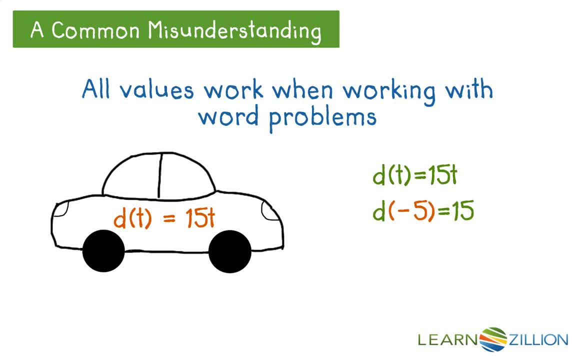 example from before and let's use an input of negative 5.. When I evaluate using negative 5 as my input, I get d of negative 5 equals negative 75.. Well, what does this mean? It means that my output the distance traveled.